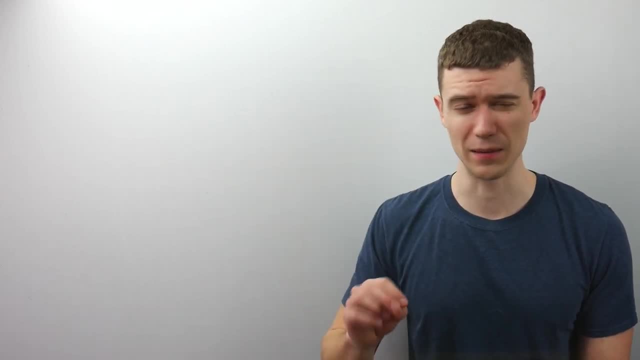 you're just writing down from the sentence- I'm assuming it's a word problem or something here- Writing down from the sentence or, if it's not a word problem, just the facts. Can you translate the problem into mathematical statements? This is often a hard thing, but if you can take things from the sentence or from the problem and 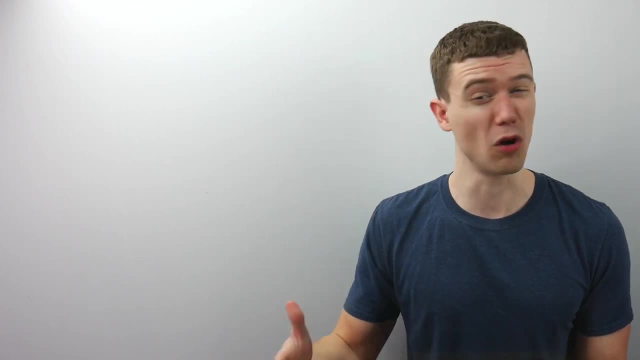 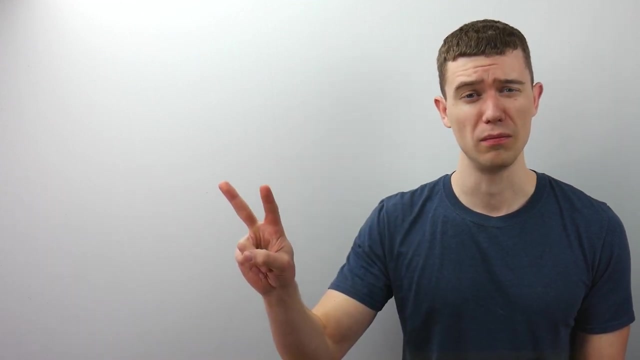 write down what that means in math. believe it or not, you're already making huge progress. So you've started. You wrote down what you know, Even if it doesn't help you solve it. Step three is: look at what you've written down. 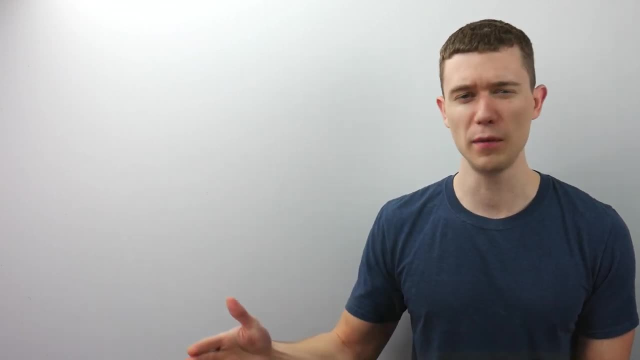 Write the logical conclusions. This doesn't have to be perfect, It doesn't have to be the correct way to solve the problem, But what you have in mathematical statements, start putting them together, or maybe just individually. They have conclusions right, The if-then kind of things. 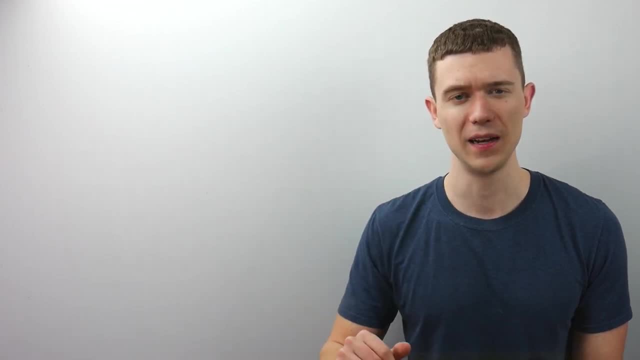 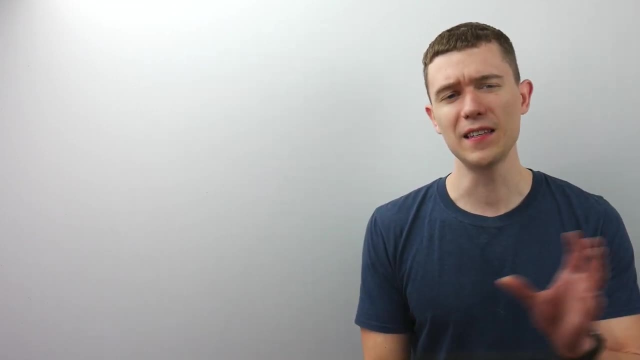 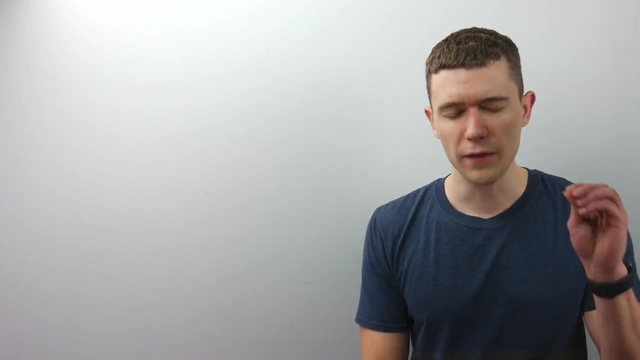 What's the next logical step Of the statement? Everything you write down, you know it should be leading somewhere. Step number four, and this is something I see many kind of earlier students run into: If you've written down what the logical conclusions are, it's time to think. 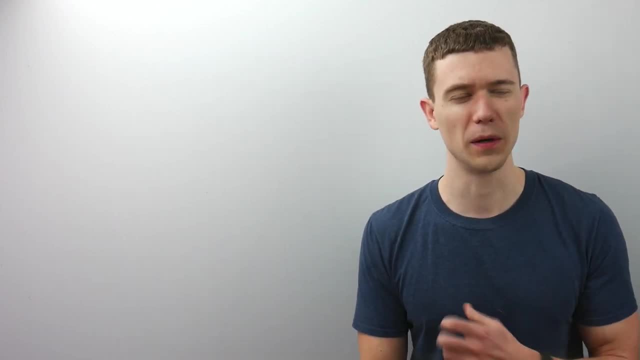 what was the question? right? You've got conclusions here, but are those conclusions really the question that was being proposed asked? right? Identify the question. Remember what does the question ask And what does the question ask in terms of mathematical statements. 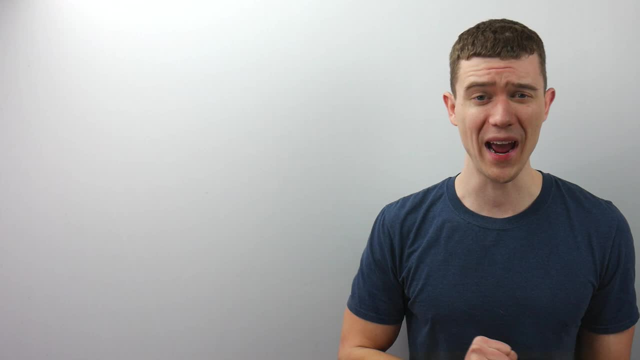 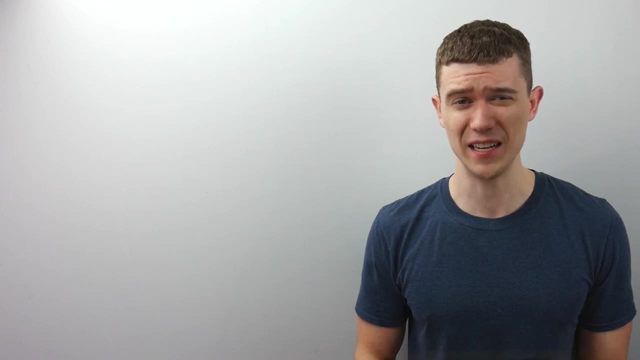 Right, Because if you can write down what you have, what the question states in math, and you can write what the question answers in math, that's really all you need. So step number four: you identify what the question is asking mathematically. Step number five: 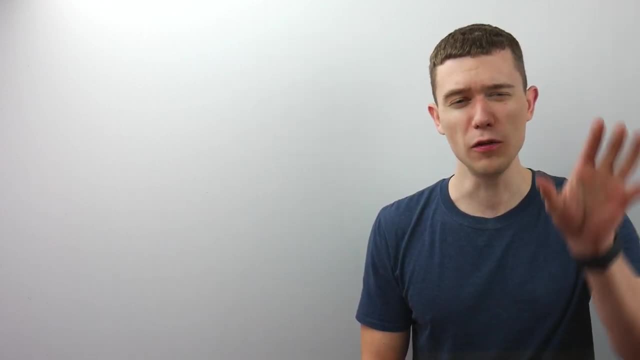 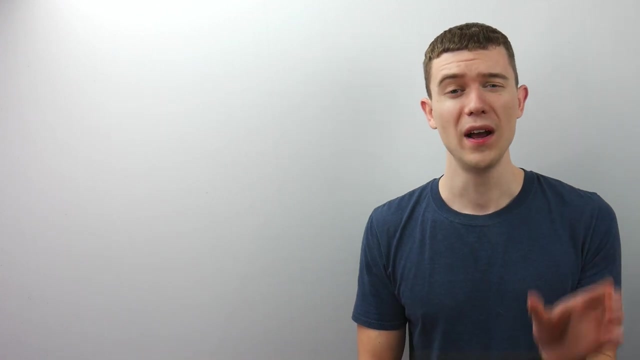 you write more conclusions, right? so now that we've written conclusions and maybe we've answered the question already, i mean you'd be so surprised how fast you get this done. but if you identify the question mathematically, you should start to feel the wheels turning. you should start to have 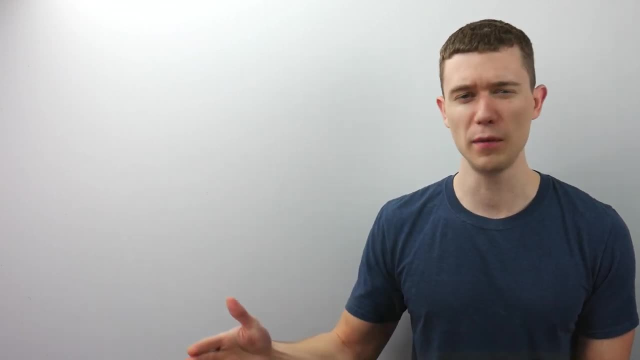 Write the logical conclusions. This doesn't have to be perfect, It doesn't have to be the correct way to solve the problem, But what you have in mathematical statements, start putting them together, or maybe just individually. They have conclusions right, The if-then kind of things. 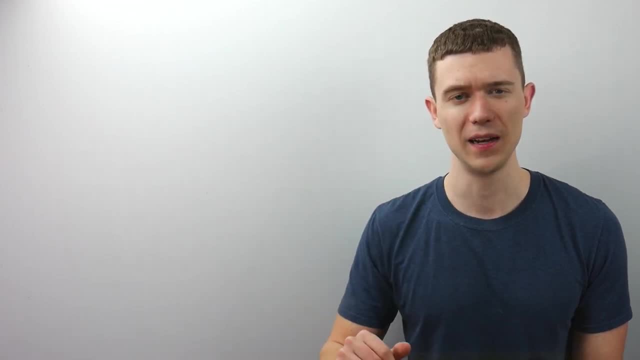 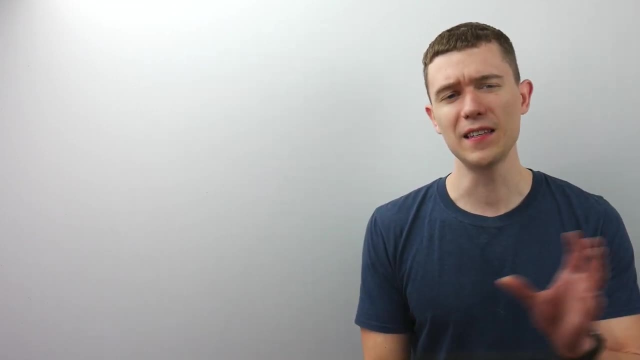 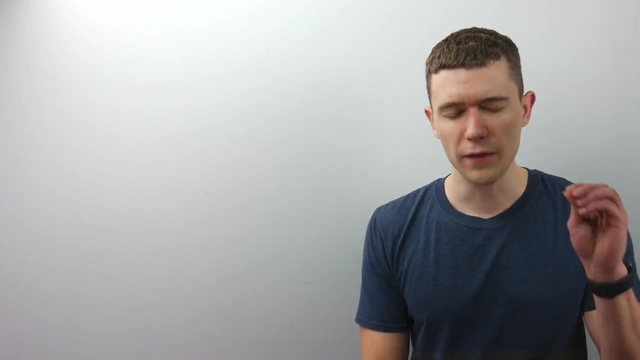 What's the next logical step Of the statement? Everything you write down, you know it should be leading somewhere. Step number four, and this is something I see many kind of earlier students run into: If you've written down what the logical conclusions are, it's time to think. 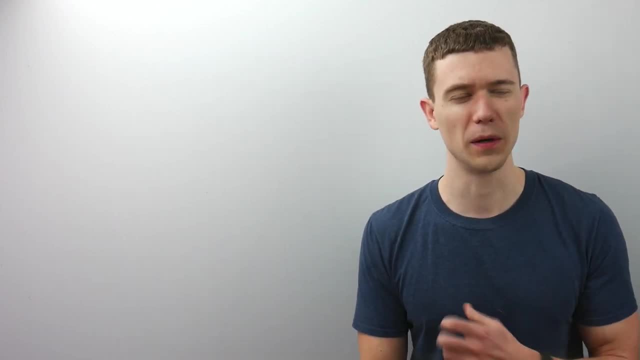 what was the question? right? You've got conclusions here, but are those conclusions really the question that was being proposed asked? right? Identify the question. Remember what does the question ask And what does the question ask in terms of mathematical statements. 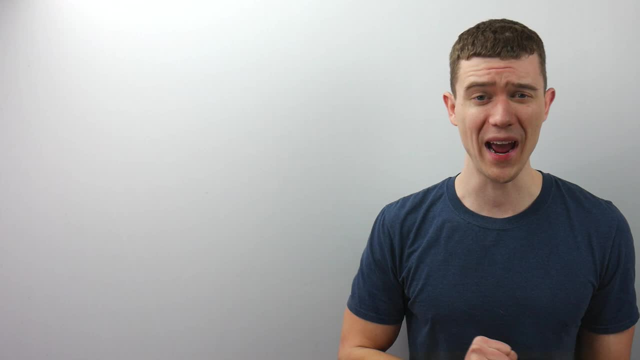 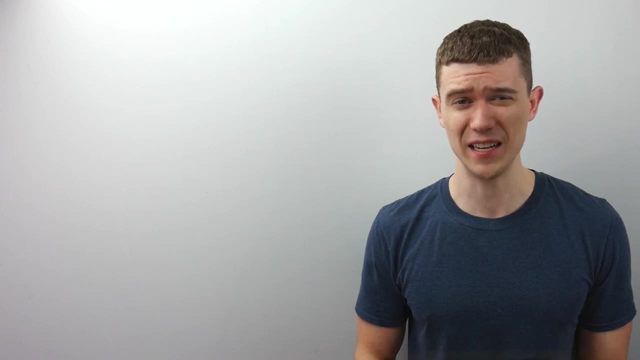 Right, Because if you can write down what you have, what the question states in math, and you can write what the question answers in math, that's really all you need. So step number four: you identify what the question is asking mathematically. Step number five: 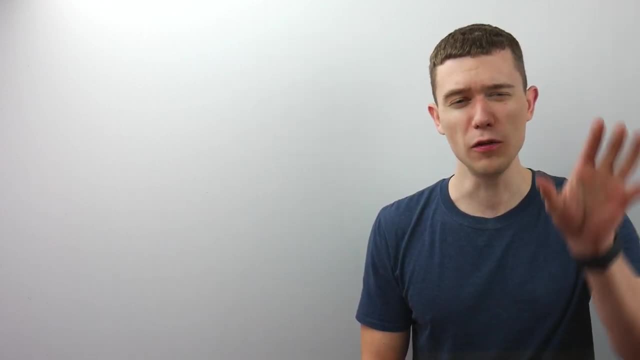 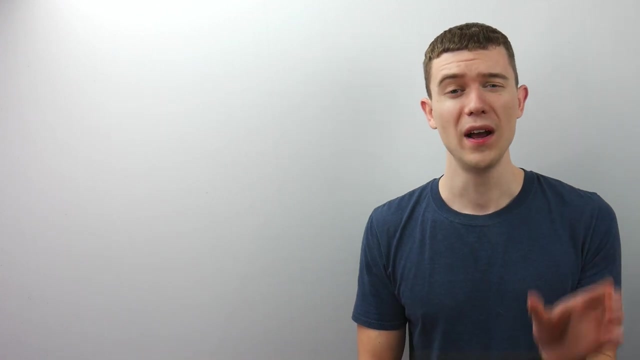 you write more conclusions, right? so now that we've written conclusions and maybe we've answered the question already, i mean you'd be so surprised how fast you get this done. but if you identify the question mathematically, you should start to feel the wheels turning. you should start to have 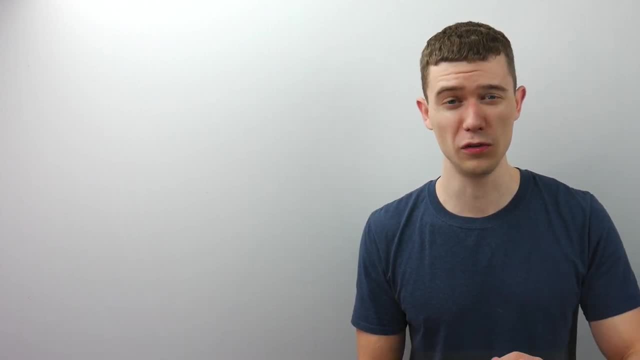 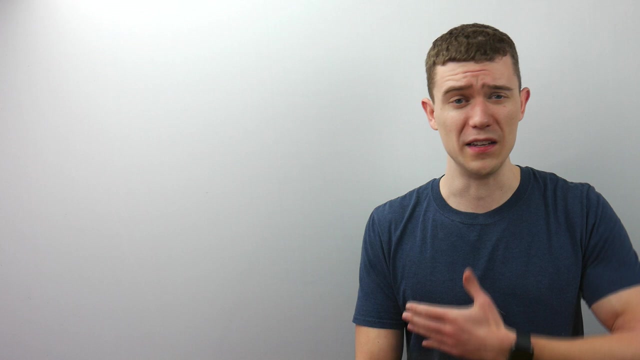 some insights and maybe you can write even further conclusions, kind of pushing the barrier even closer to answering the questions, because step six is just to solve the problem. once you've done this, i mean you should pretty much be there. i mean all you've done is you've written what you have. 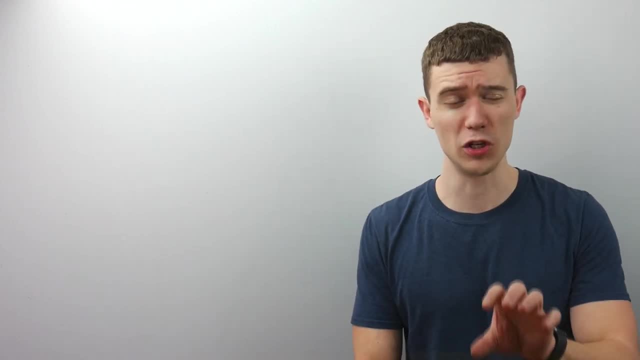 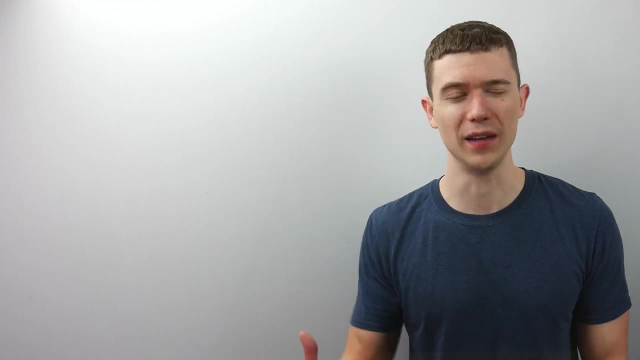 you've written what you want, and you've written things to connect what you have and what you want. i mean, that's all we're really doing here. that's what we're doing with nearly any math problem. now i'm really describing how math proofs are written, but this works for lower level concepts too. at 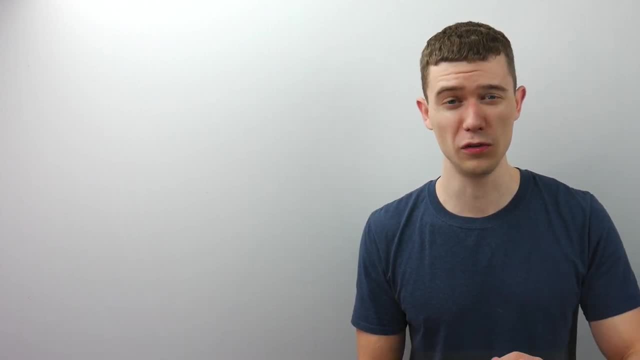 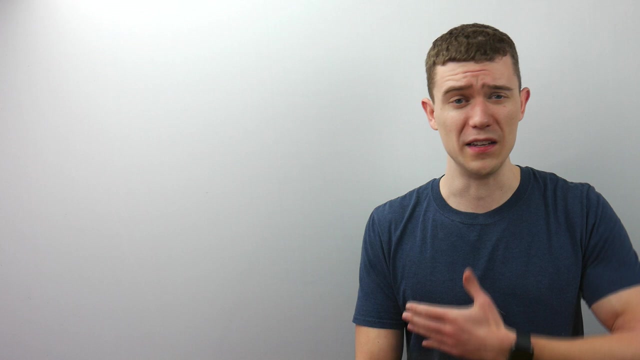 some insights and maybe you can write even further conclusions, kind of pushing the barrier even closer to answering the questions, because step six is just to solve the problem. once you've done this, i mean you should pretty much be there. i mean all you've done is you've written what you have. 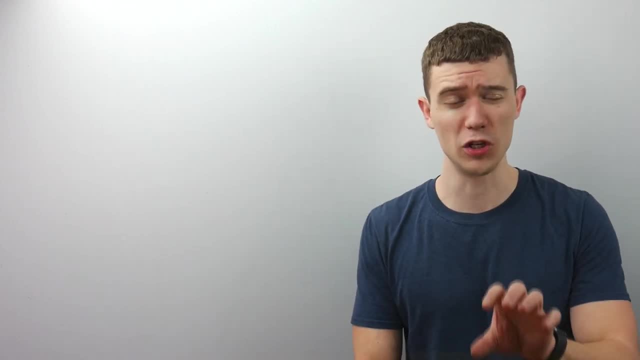 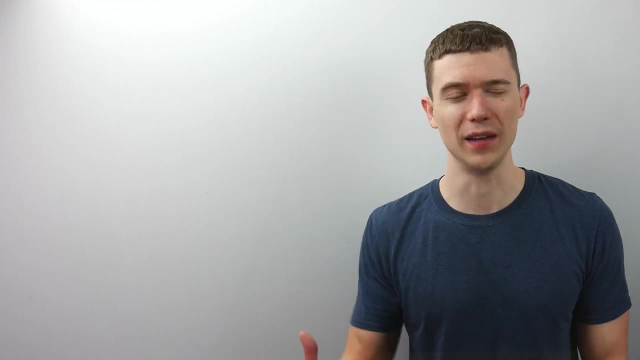 you've written what you want, and you've written things to connect what you have and what you want. i mean, that's all we're really doing here. that's what we're doing with nearly any math problem. now i'm really describing how math proofs are written, but this works for lower level concepts too. at 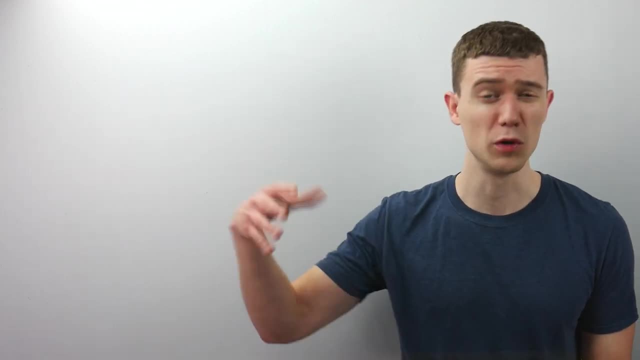 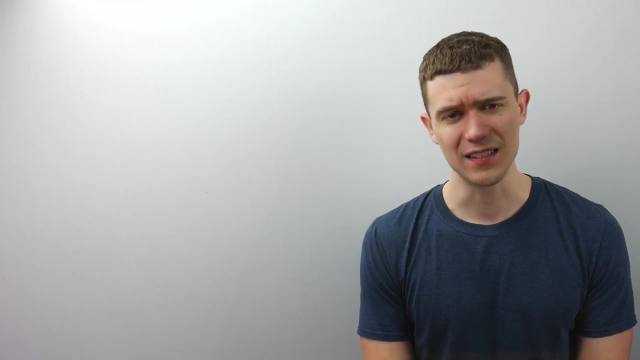 least in my opinion, you now here's the thing, step six here, which was solved the problem. you might not be at step six yet. you might not. you might have done the first five and say, well, i can't solve it, i still don't know. step six, subsection b, is you walk away? yeah, you walk away from the problem, because this is a. common phenomenon. you may have heard of this sort of thing happening before you. you want your brain to just turn off. stop stop working on the problem. go do something else. do something relaxing you. let your subconscious brain start working on the problem. it's the way that it works. you ever hear of having like insights. 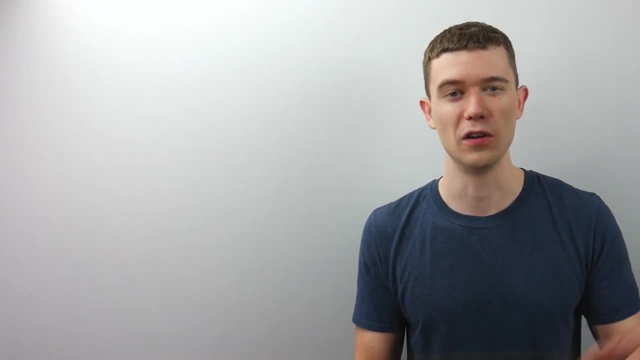 in the shower, you know, when you weren't even thinking of it, like people, you know they have a. this is a famous thing, i believe people, people talk about it. i promise they work on hard. problem, they can't figure it out. they go take a shower. you know, their mind drifts off, drifts off and all. 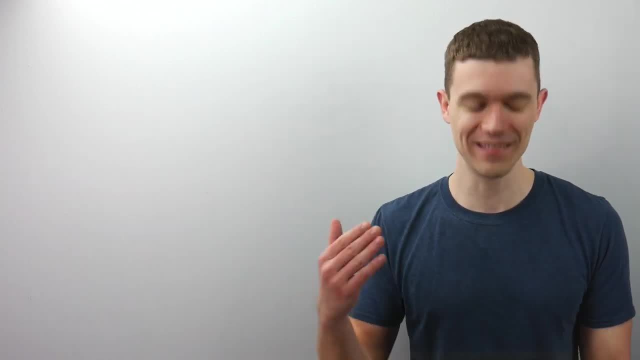 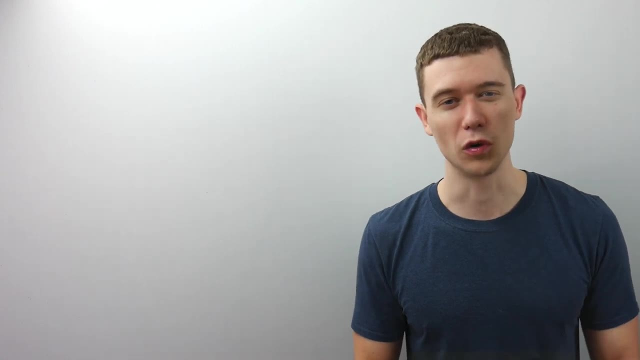 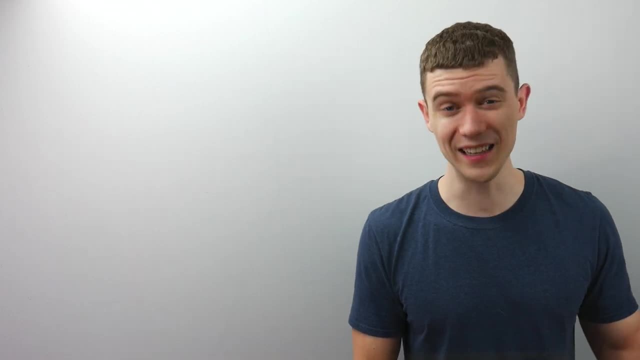 there are my steps again. so there are my steps again. so there are my six steps for how to solve, six steps for how to solve six steps for how to solve any problem at all, or at least at least most math. any problem at all, or at least at least most math. 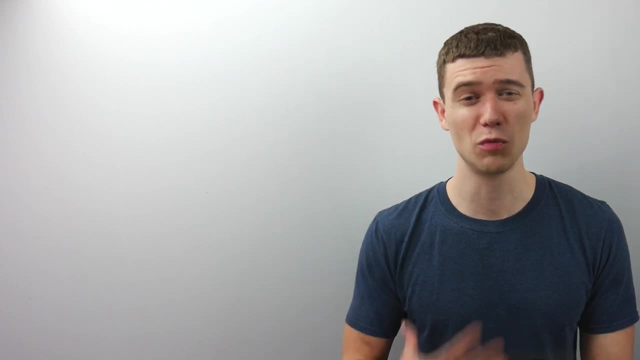 any problem at all, or at least at least most math problems. i don't know if it's a perfect list, but problems. i don't know if it's a perfect list, but problems. i don't know if it's a perfect list, but i think it's worked well. for me. this is sort of 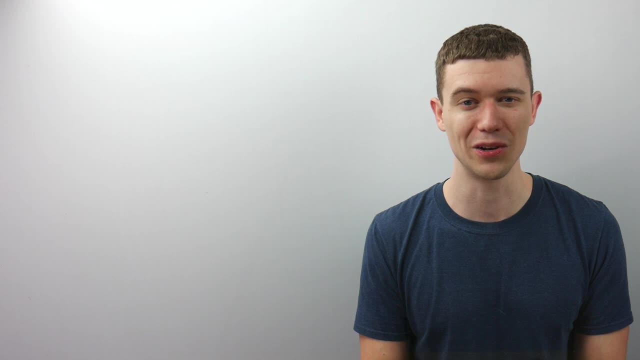 i think it's worked well for me. this is sort of i think it's worked well for me. this is sort of how i tackled things, especially in grad school. how i tackled things especially in grad school. how i tackled things, especially in grad school, when i didn't really know how to solve. 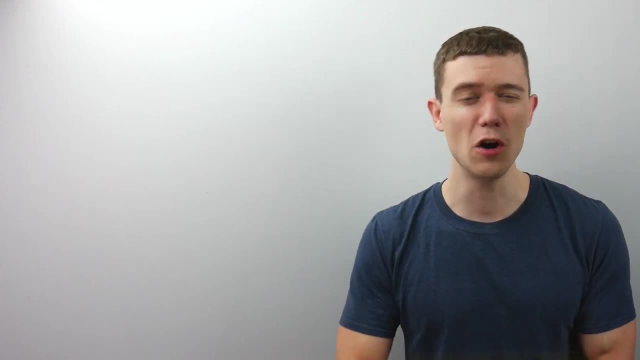 when i didn't really know how to solve, uh, a problem. so much so i hope you enjoyed the list, i hope it you. i hope you use it well, you know, i hope it helps you out. i really appreciate you watching the video until the very end, and i hope you have a great day.